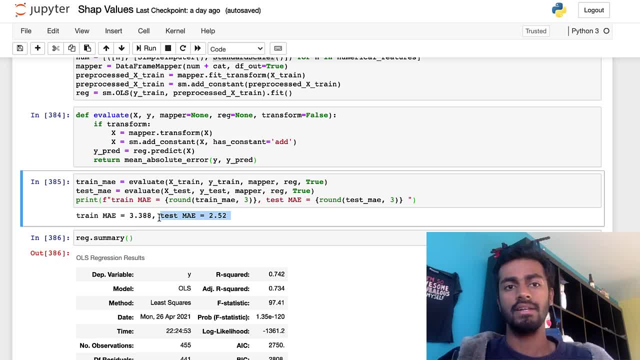 evaluation metric And I get a pretty reasonable amount right here. That's great. But now, let's say, I want to do some model interpretation, understand what is contributing to this And what are the most important features, And so I use stats models and try to come up with this summary table over. 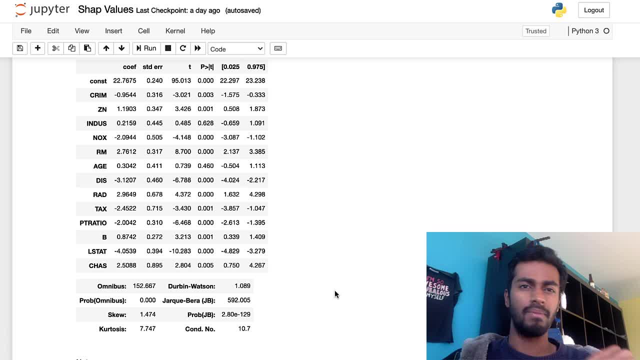 here And in this entire pre-processing step I did some standard scaling and yeah, so they have mean zero standard deviation one. And at this rate I can look at the coefficients and kind of look at this and say, well, this is equivalent or proportional to the feature importance, as long as they are significant. 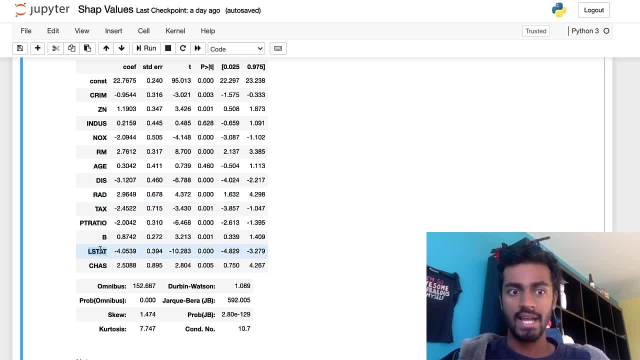 coefficients, So some significant values here will be, like L stat, which has a very high magnitude value compared to the rest, And this would be like one of the most important coefficients, closely followed by probably this dis right And so on, which this is reasonable to say, reasonable. 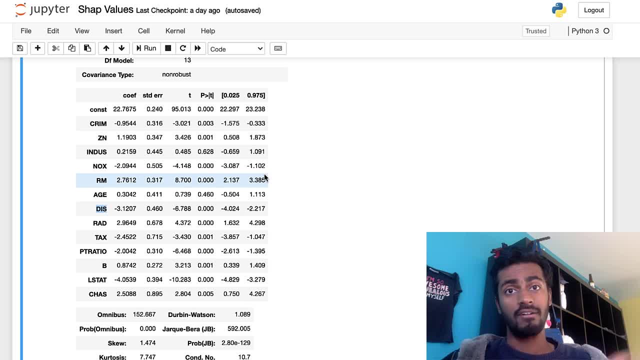 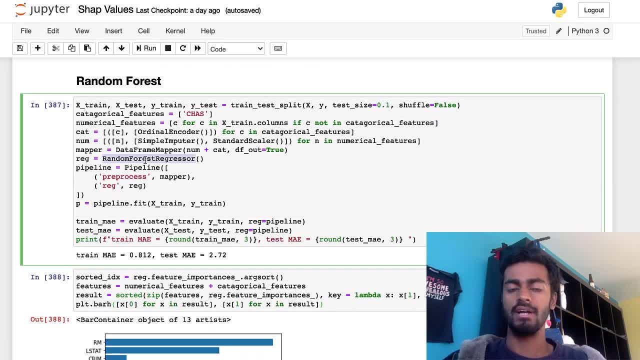 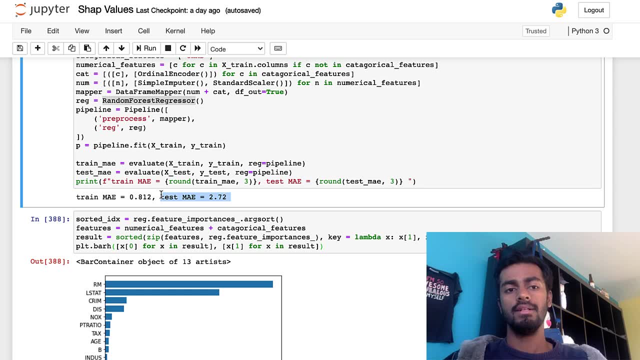 create a random forest regressor, right. So the only thing that changes here now is like adding a random forest regressor. all the pre-processing steps remain the same, and I get another test, ma e, which is pretty reasonable too. And when I look at the feature importance here, though, 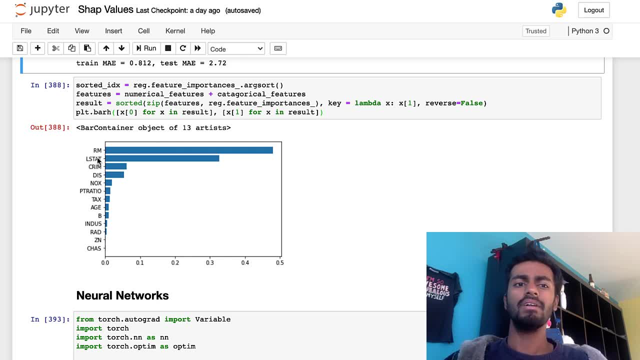 I kind of see something similar L status still up there, But it's it's a little similar, a little different, not too not too crazy different, But but yeah, in general it is a different way of assessing feature importance, because here I'm using a build. I'm using a build component versus a. 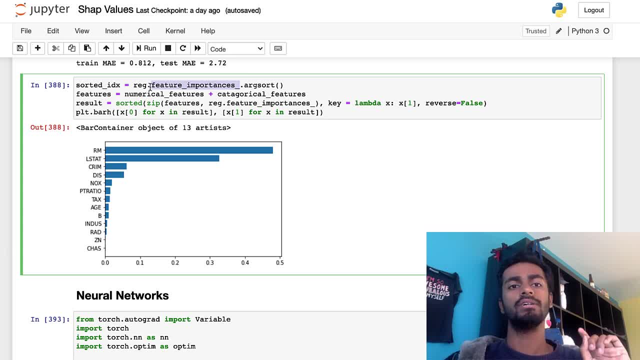 in method call right here, which essentially determines feature importance depending on the node impurities of the tree that's constructed. yeah, and this is, though, very specific to these tree based algorithms. but let's say now I want to change it from random forest regressor to a neural 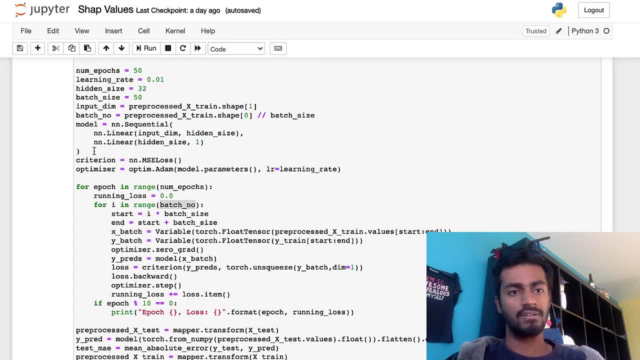 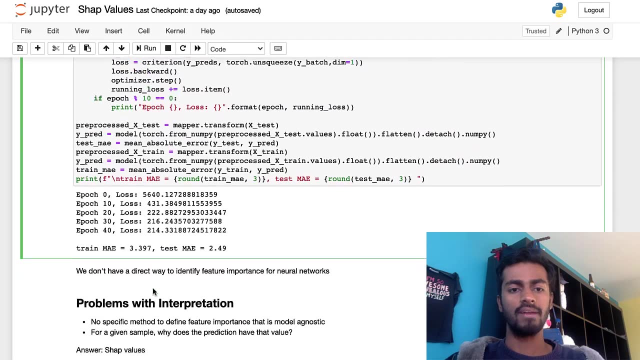 network where now I'm like flushing out a neural network architecture right here. I'm building with PyTorch, by the way, and so I have one hidden layer with an output layer. no activation functions here and I'm using mini batch gradient descent to process all these batches. and when I look at 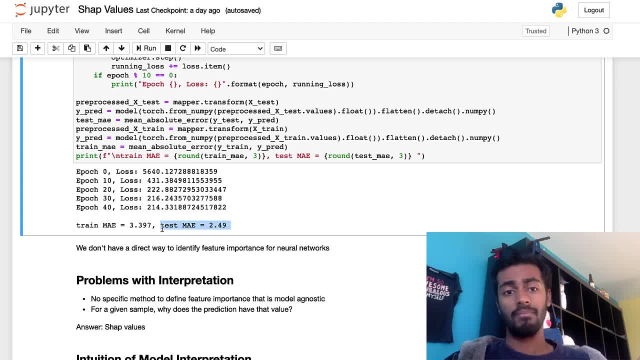 my test nae well it still. it performs really well, probably better than all the rest right here because of its ma, but unfortunately, though, I don't really have a direct way to identify feature importance of a neural network, not with like a built-in function that I can just visualize at. 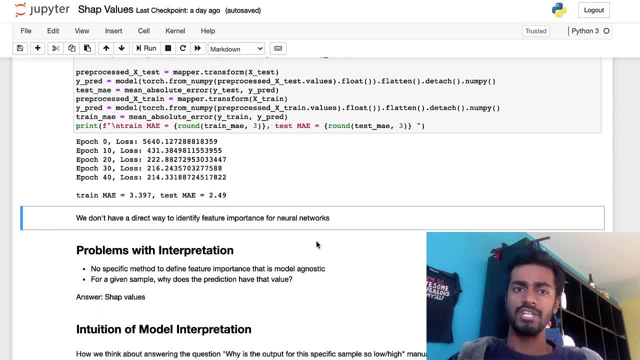 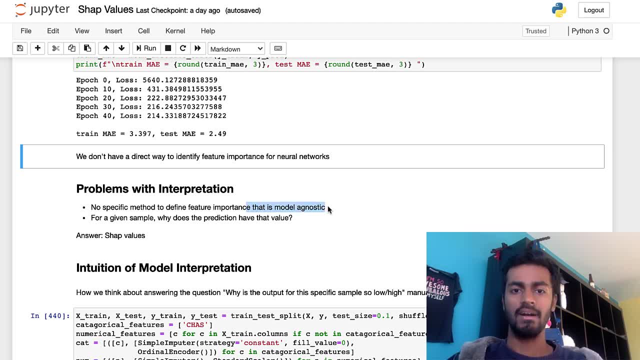 least as far as I know right now, and on top of that in general, these: when looking at all these three methods, I don't see like a single way to define feature importance that is model agnostic, so one way that I can just feed any kind of model in order to get a feature importance for well, these for every feature and on top of 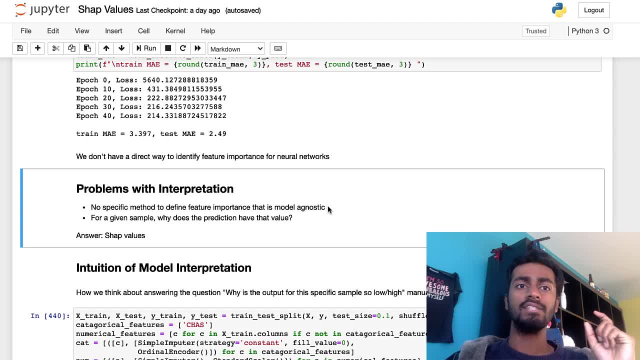 that. what if I want to know, like for a given sample, why it's predicting the way that it is, like, what is contributing to a specific samples prediction too, and not just feature importance? well, all of those, honestly, can be answered using Shapley values, and we're going to be taking a look at that later, but before that, 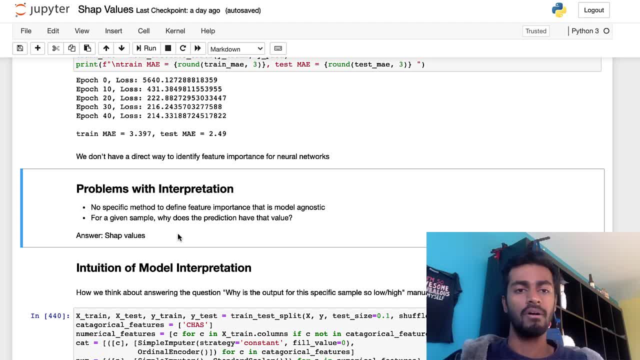 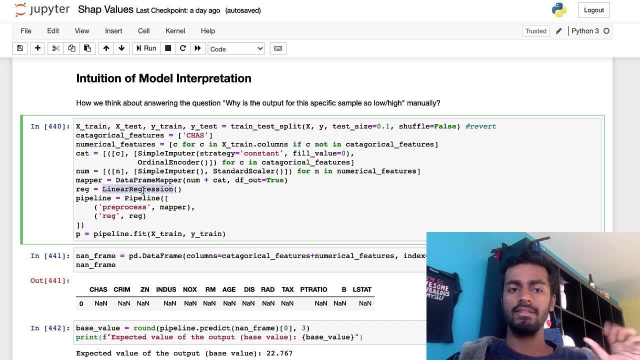 let's take an intuitive look at how we would intuitively interpret models. now. let's think about this for a sec. okay, let's first reconstruct our linear regression model. we have it. that's great. let's pass in now a non-feature data frame, basically a data frame of just Nance for all. 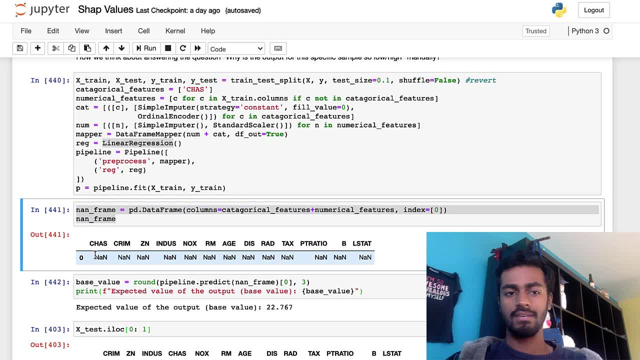 the features and let's see what our model outputs. now, obviously, with all these Nance, they're going to be imputed by your simple imputer, right here, which is going to, well, right here actually, which is going to, by default, imputing the mean value of. 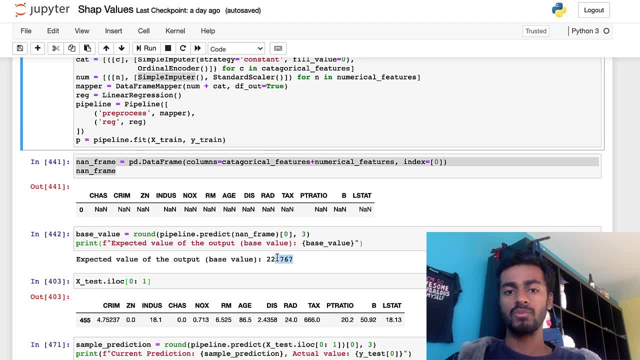 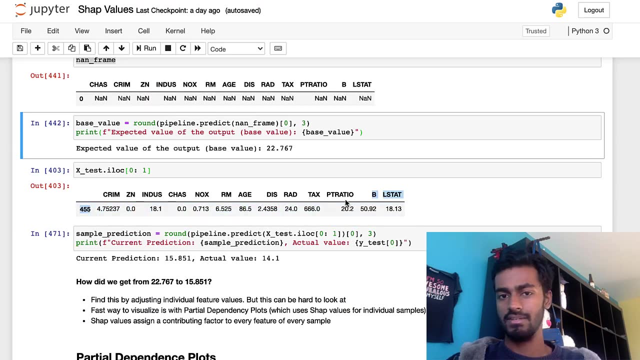 those features and when we do, we get a model output of 22.767 and this is, you can say, the, the expected output of the model or the base value, more technical terms. now let's just take one of our test samples- I'm just taking the first one right here- and this is how the data frame. 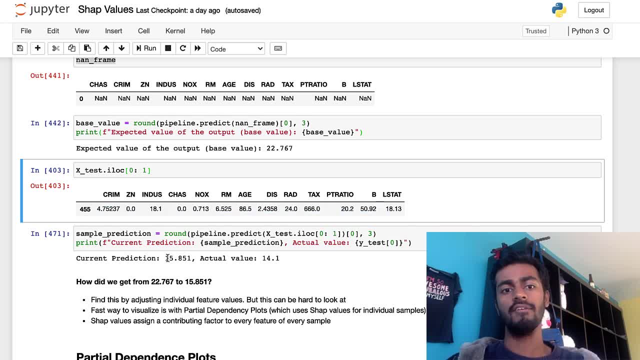 sample looks and we throw it into our model and it makes a prediction of 15 point eight five, one which is fifteen point eighty five. one thousand dollars is the median house price. that's fine, but how do we get from this twenty two thousand right here, or twenty two point seven six? 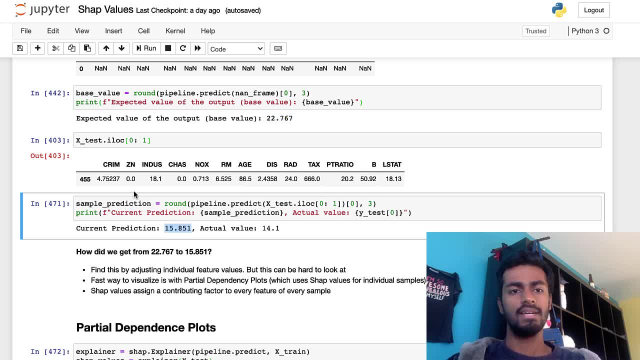 seven all the way down to fifteen. point eight, five, one. it's because of these features. right, but how do I know which feature has contributed how much? well, the way I would probably do it is just first take one feature at a time, like crime, and then try to vary it up and down and see how. 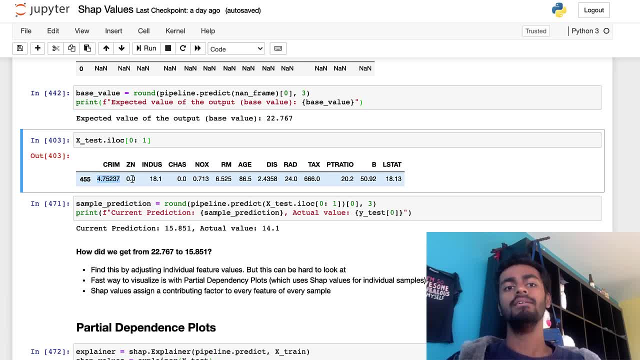 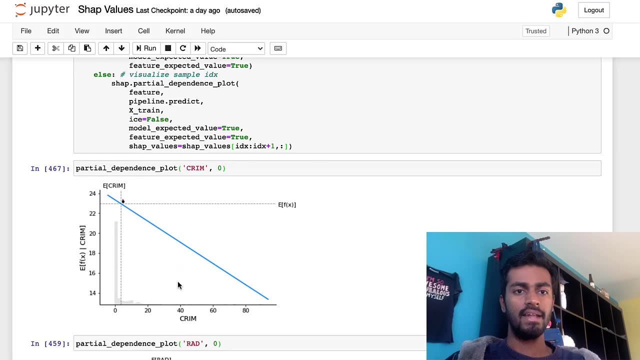 the model output varies with, you know, varying crime same. do that with ZN. how very this. see how the output varies. um, a good way to visualize exactly this is using partial dependency plots. so I'm going to construct a partial dependency plot right over here and for crime, for example, it's exactly what. 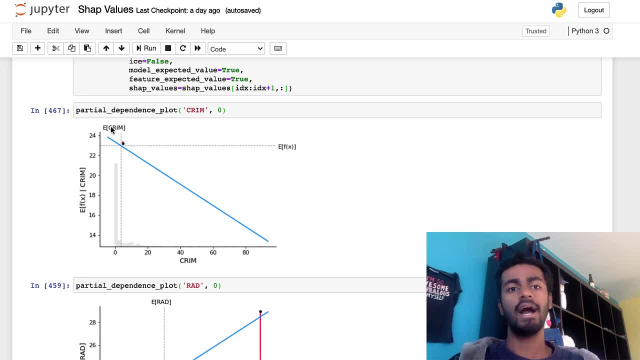 I mentioned. the x-axis is the feature crime and the y-axis is the model output, as we vary crime when we're given crime. so, um, this gray data frame- I mean this grit, not with data frame- this gray histogram over here is the distribution of all the test samples, the crime of the of these. 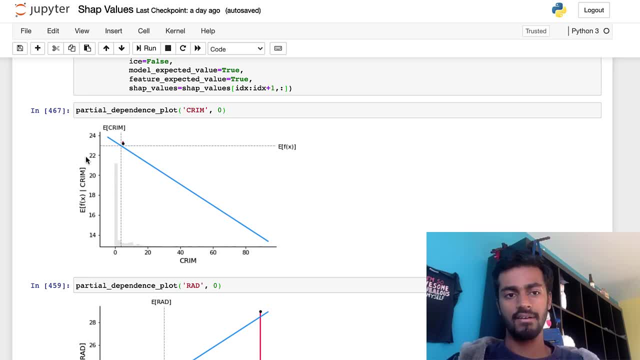 test samples. so you can see that they're all pretty low over here and the crosshair is the expected values. so this cross, this line, is kind of close to like twenty two point seven. um, you know around that value, at least it's dependent internally there's 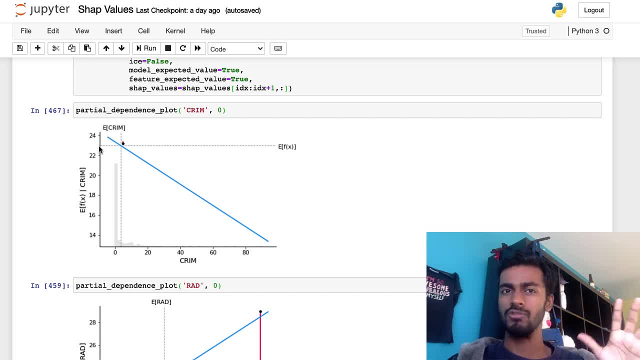 like an internal logic for computing this, so it might be slightly different, but it's around 22.7 that we discussed and the corresponding crime. right here is the kind of expected value of like which teacher is named. it just to be particular version of machine learning. in reality, all this, 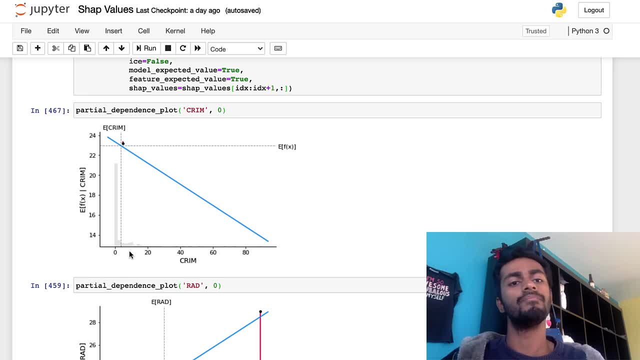 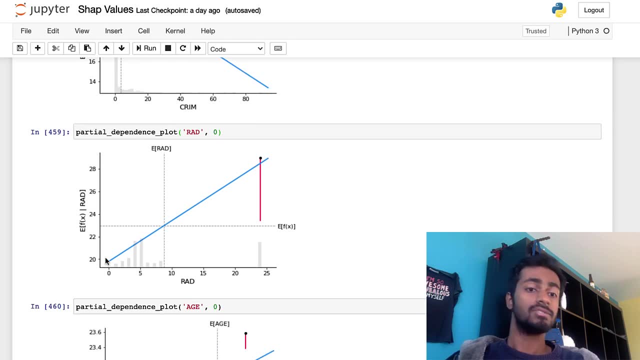 property is internal logic which shows you that if you one take an repay rate value of 10, this feature crime right here. right, Ignoring the red parts for now. So you can see that we have the same for partial dependency plots for rad. So as the rad increases, you can see that. 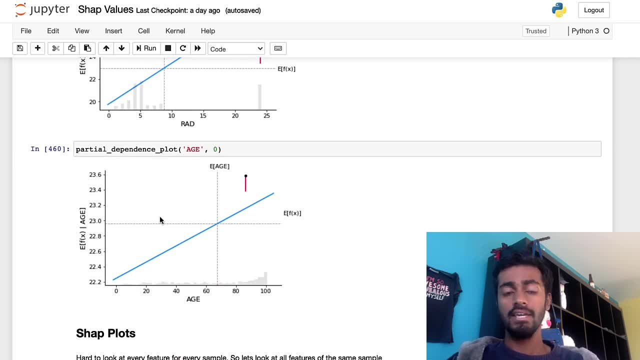 the model, output increases As age decreases. well, the expected value also increases. But you can see that the y-axis is kind of small. This entire area is not even going to increase it by like 1.2.. So although age is a factor and is proportional positively, it's not really that. 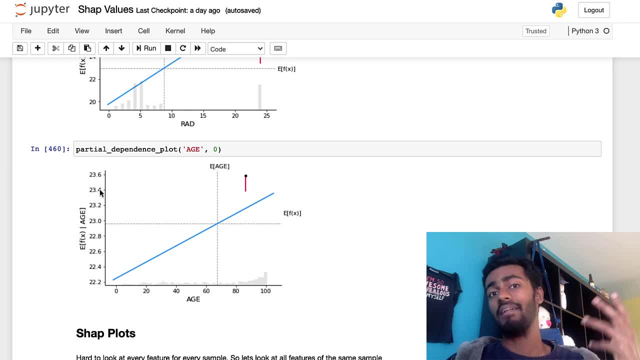 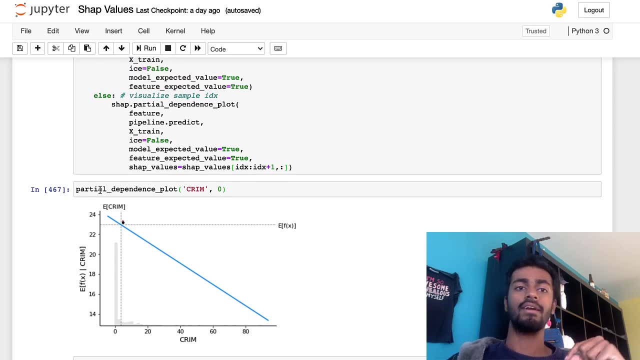 significant. So no matter what age is, it's not going to affect the model output that much right Now, looking at the individual samples. so let's say I want to look at it. you know, okay, the effect of a particular sample on the model output. well, that's where these red lines and 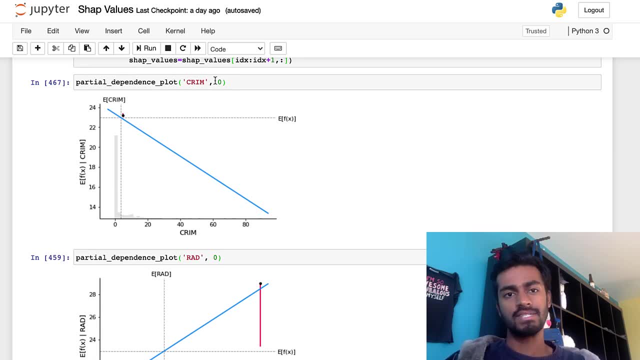 the black dot come in. So for this, you remember, I'm taking the same exact sample that we saw before. So for this, you remember, I'm taking the same exact sample that we saw before. So for this, you remember, I'm taking the same exact sample that we saw before. So for this, you remember. 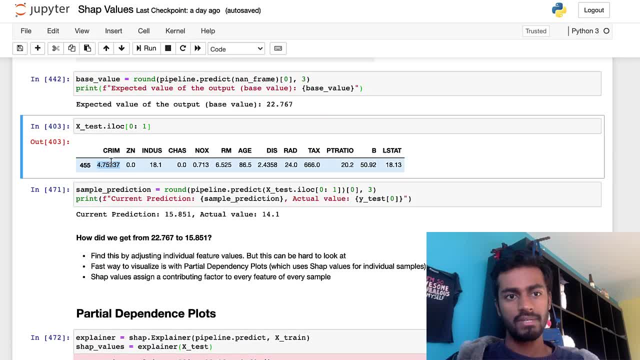 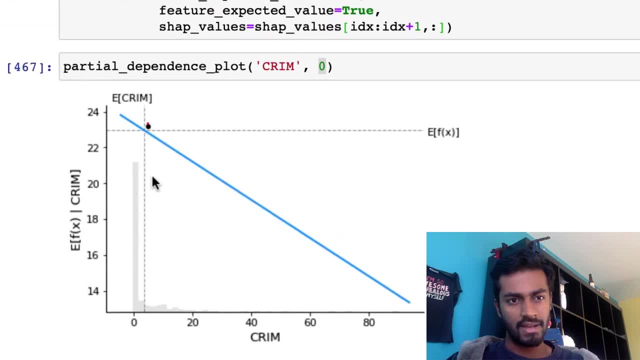 before where the crime was 4.7,. if you look here, 4.7 was that right? And if you look at the x-axis, that corresponds to this part right here and you can see it's a long 4.7.. 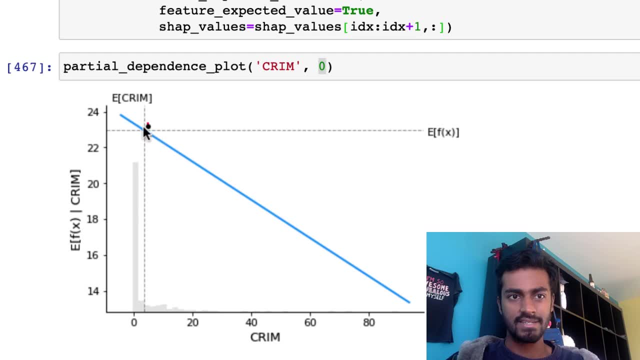 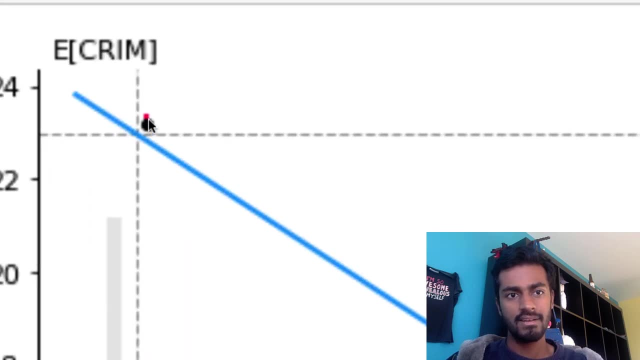 But the y-axis. of course, I don't know why that this dot is actually mispositioned. This dot should be on the blue line and the top part of this red line right here. this part should be on the gray line right. 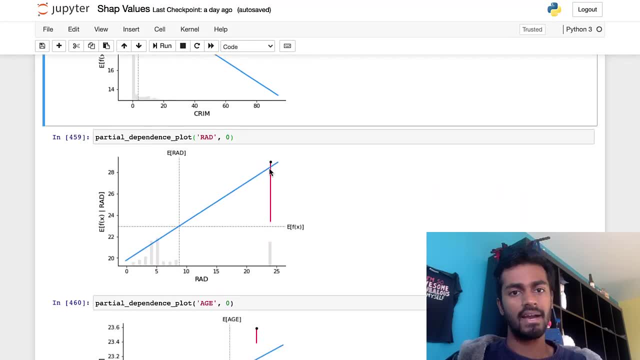 Maybe it's a lot easier to see with this example. yeah, It's also shifted up. This dot should be on the blue line. This bottom part of the red line should be on this gray line. So for this particular sample, the same sample. 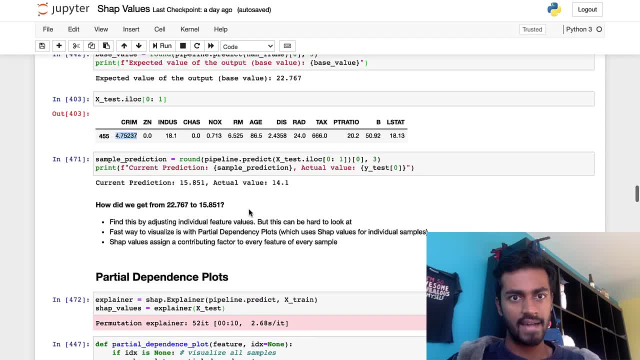 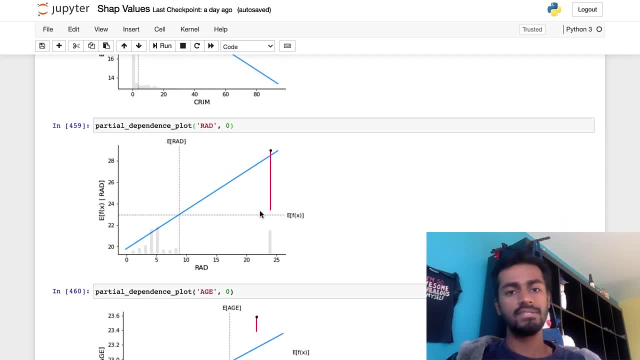 the rad was 24, and you can visualize. we can see that just by going up here. Rad was 24,, right up here, right. So plotting this out, you can see that the difference in the model output from the expected value. 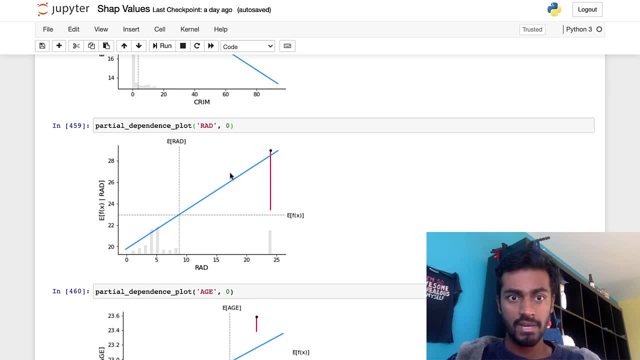 it is now like something like 27 or 28.. So it has a huge effect on the model output, increasing it by like three and four, four and a half, I don't know- something like not four and a half, it's like 22.5 plus something is 28.. 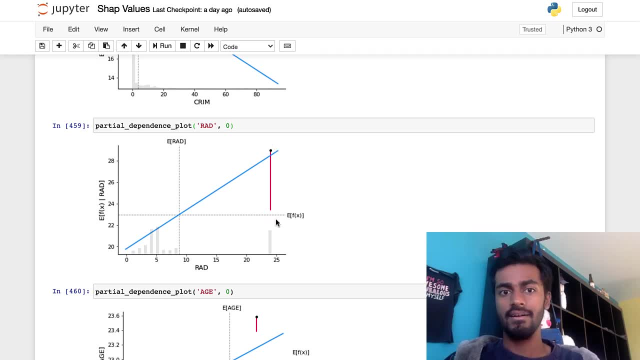 So it's like five and a half or something like that, right, And this entire value, this length of the red line, thus becomes the contribution of this particular feature, rad by this particular sample zero right, And we call this red line. 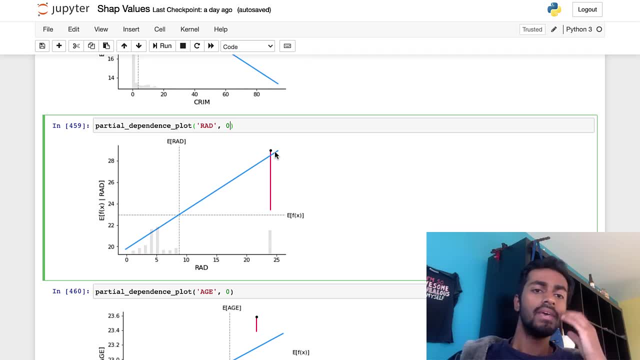 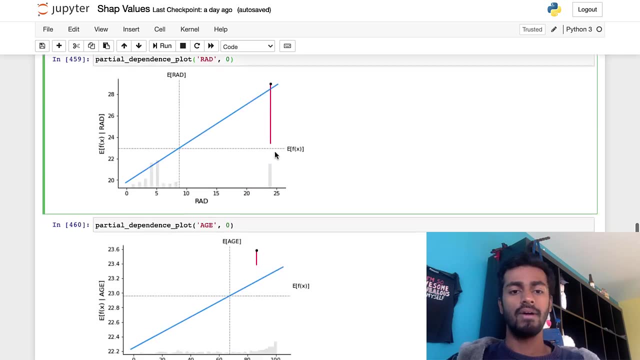 or the magnitude of this red line, the Shapley value. And so we can have Shapley values for every sample, every feature of every single sample in our entire data set. So I can keep plotting plots like this: The length of this red line is again another Shapley value. 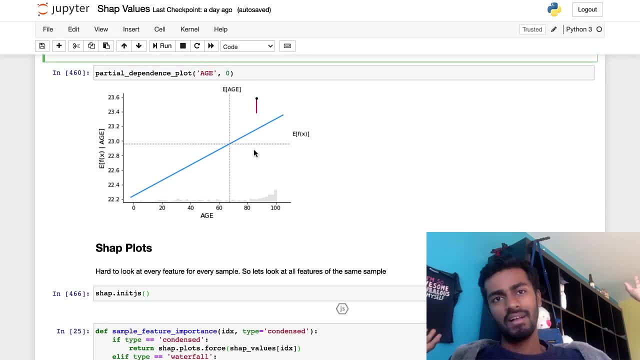 But this: it kind of gets hard to plot. so many plots for every feature, every sample, And so let's say that for every sample I want to plot it, I want to know all of these red lines for every single feature, for a particular sample. 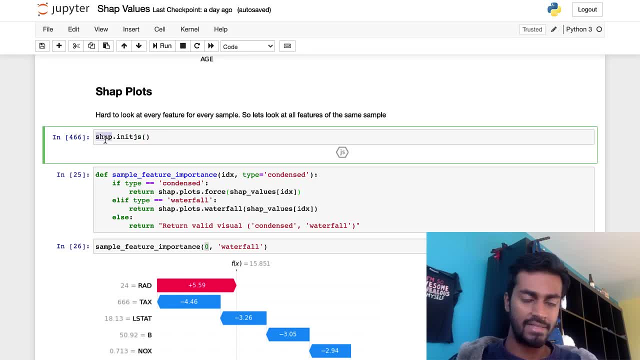 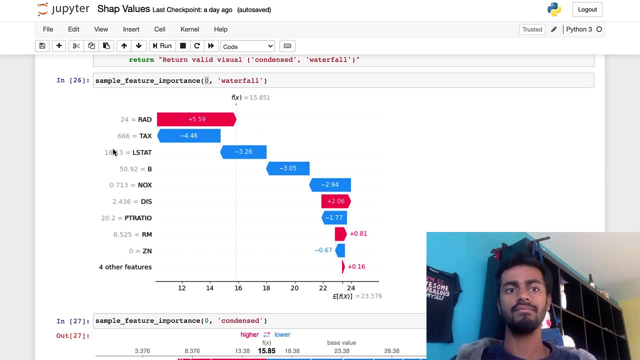 And so we have representations from Shap, the library in Python that provides exactly that. I'm looking at the same exact sample right, Remember 24 rad. we saw that before right, And I am going to plot it for every other feature, though, right here. 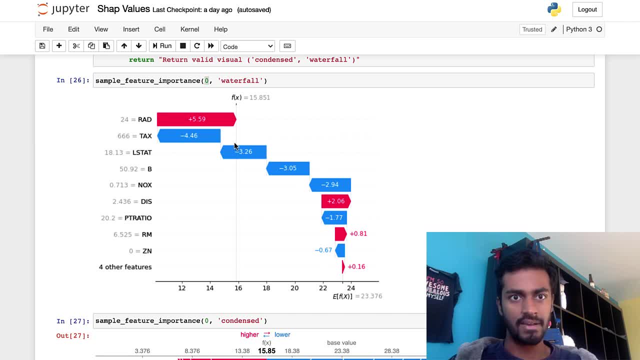 And you can see that this gray line, there's like a little gray line that's going up here, And it says f of x is 15.851.. That is the model output, And the expected value for model output, though, is 23.376. 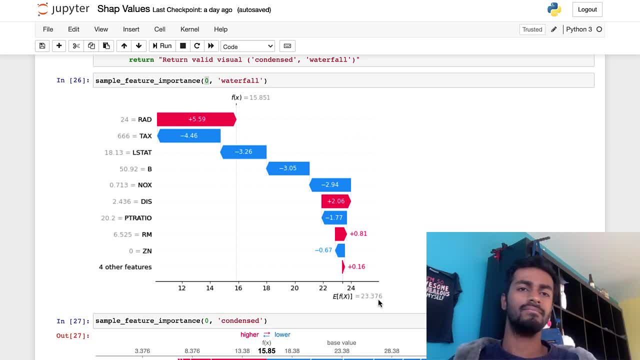 We determined it to be like 22.7,, but you know, internal features of like Shap kind of have determined it this way, which is similar, And so the difference between these two is negative 7.5.. How did we come up with? 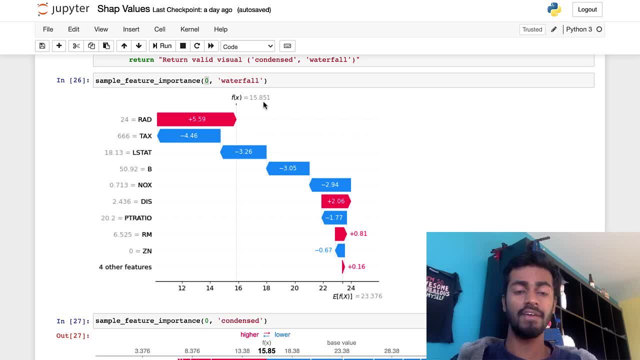 how on earth did we get from 23 here to 15.85 here? Well, it's shown by every single feature right here. So it looks like rad had a huge impact by increasing you know, having a positive influence on you know. 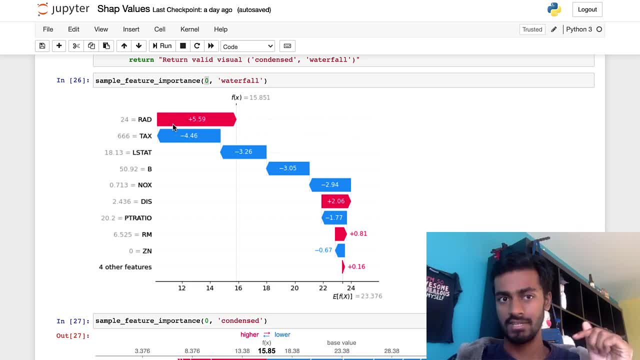 increasing the prices of specifically for this specific sample And then the tax lstdb and nox had a good impact in bringing down. you know, increasing the prices of specifically for this specific sample And then the tax lstdb and nox had a good impact in bringing down. 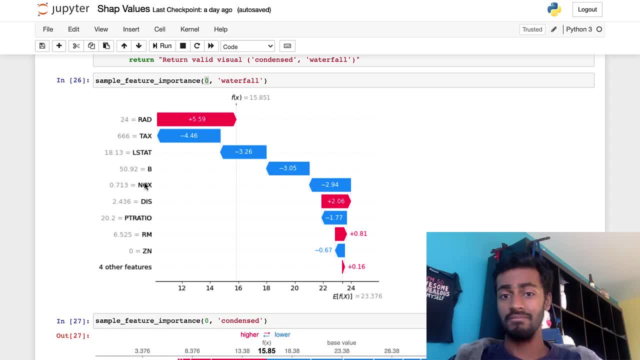 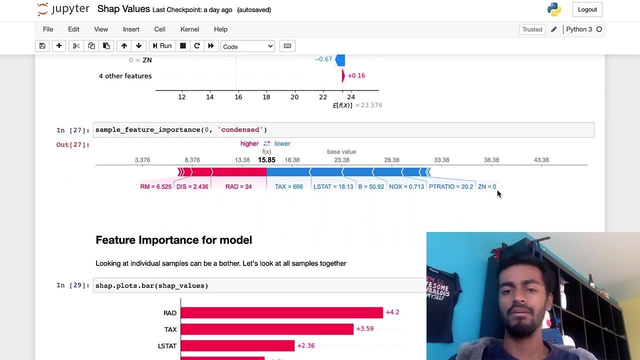 the entire price, And so we're able to visually interpret why exactly this specific sample is given an output of 15.851.. Now, a cooler way to like. I like seeing a condensed representation. It's exactly the same pieces of information, but just not in a waterfall model. 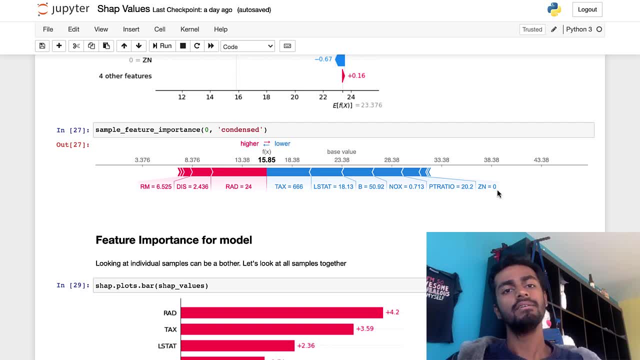 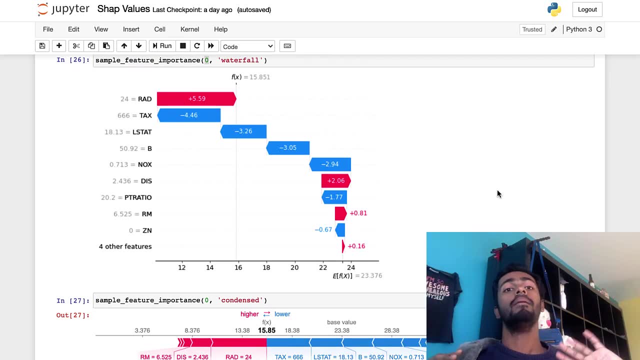 Sometimes this is easy to look at whatever you feel is comfortable. So now that we have- yeah, this is for an individual sample, though- But what if we want to bubble this up to determine model importance? Well, all you need to do is take all these shat values. 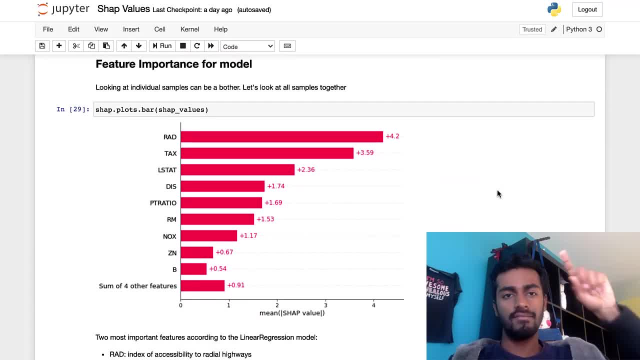 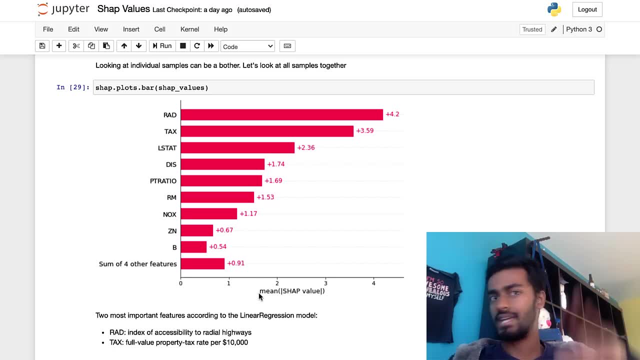 for every single feature, in every single sample, And for every single feature column, we are going to just determine the mean of the absolute value, of the Shapley value. So, column wise, just take the mean of the absolute value, And so you end up with a plot that's like this: 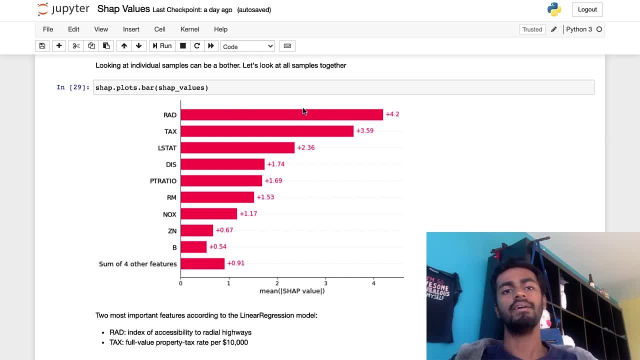 where the Shapley values would be proportional to contribution right. And so we can see that, for again, this was a linear regression model. Rad is the most important feature, followed by tax, followed by lstdb, followed by this, followed by P ratio, and so on. 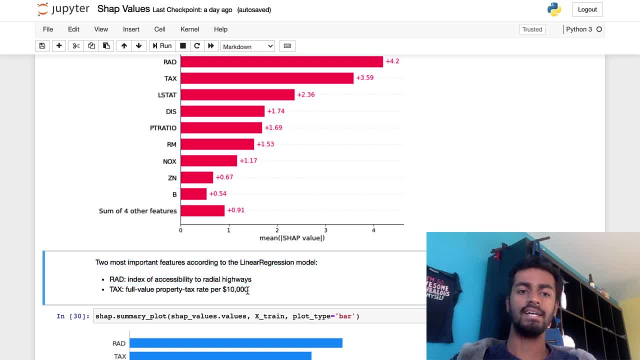 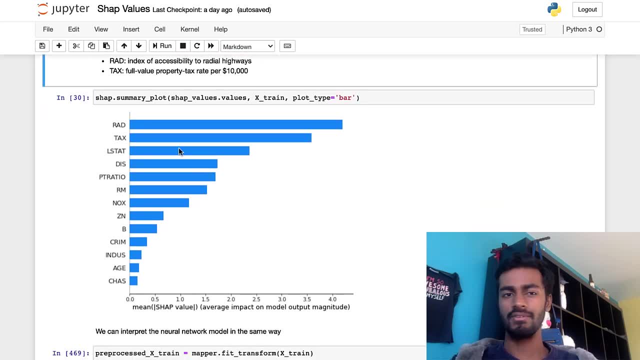 right, And so that's kind of why I have like a note over here that says, like, what features are important to this linear regression model? Yeah, this plot is kind of the exact same thing. It's going to give you the exact same information. 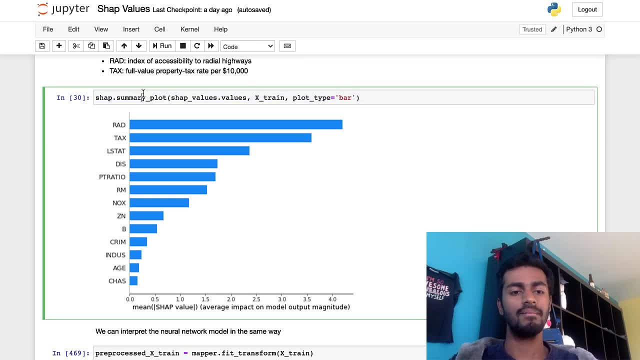 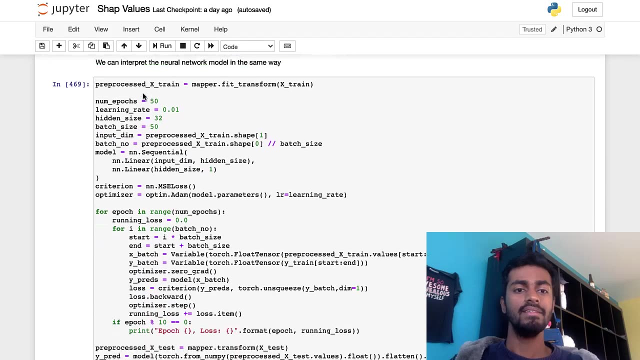 It's just a standardized way of plotting it out. That's all Okay. cool Now that we have a linear regression interpreted, even if I wanted to replace this entire network with a neural network. sorry, this entire model with a neural network instead. 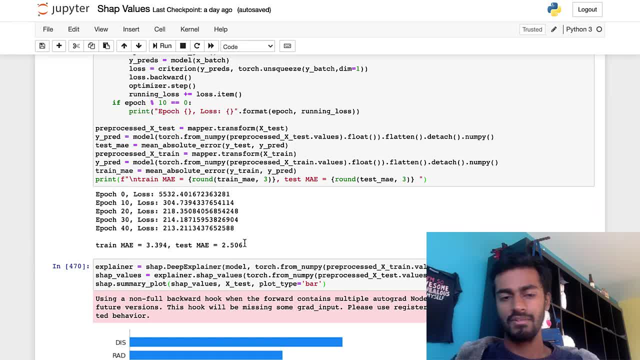 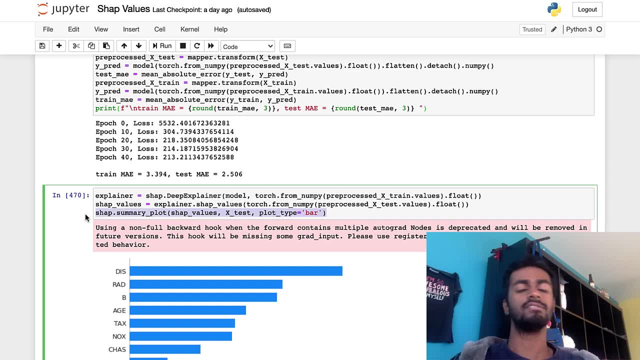 this is the exact same code that I showed you before, And we're getting a very similar MAE. Yeah, And now I can just create a summary plot, which is basically: you know, determine the Shapley values and then aggregate them across every column. 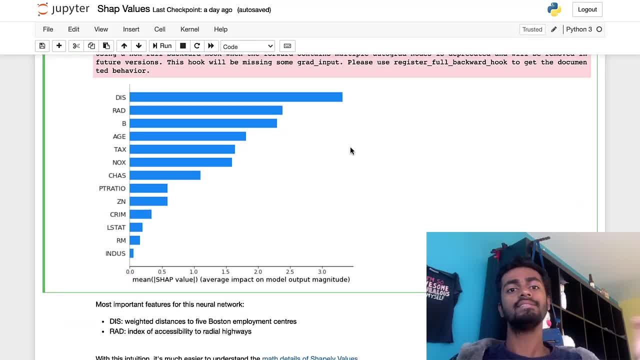 And you get well, feature importance. And this is a very standardized way so that you know, for any model that I want to create and any model I want to interpret, I can, And I can also determine it for every single sample. 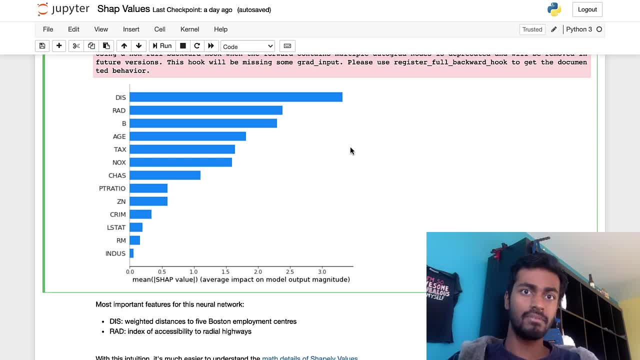 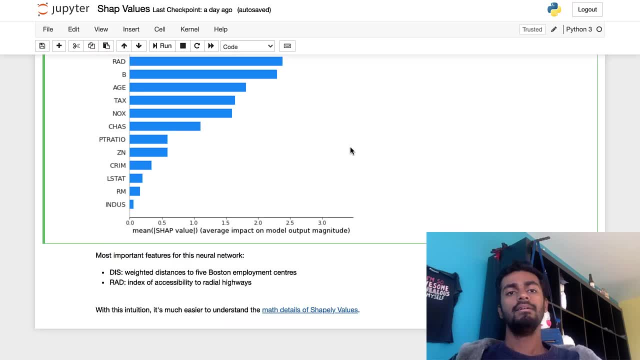 I can determine the contribution for every single feature in that sample, or for every single feature I can determine, you know, the feature importance across the entire data set. So, yeah, that's actually the good basis of Shapley values There are. 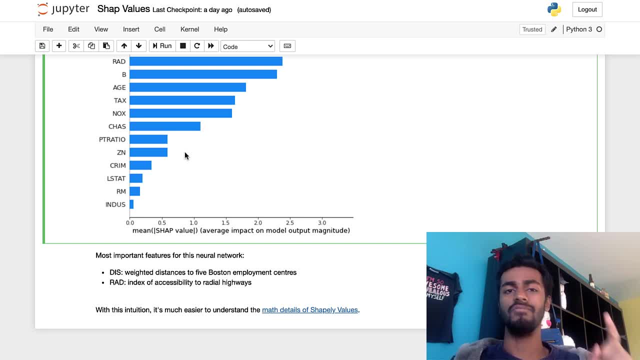 there's a documentation for Shap, which is the main library I used for creating the Shapley values. I will link that down in the description. but now, armed with this knowledge, I think it'll be easier for you to understand exactly the math. 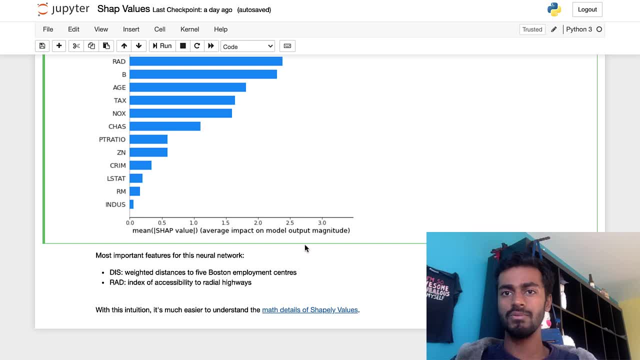 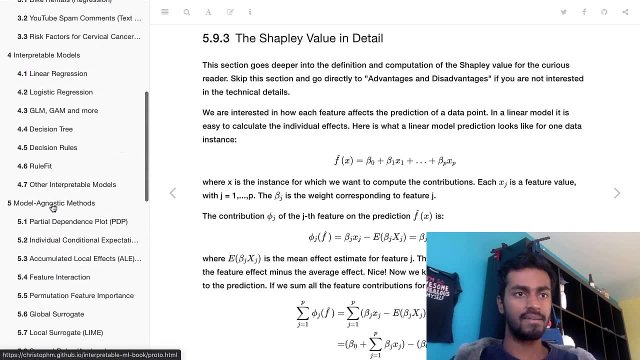 the mathematical takes on Shapley values that you see in documentation. I've linked to it in here below And if you click that it'll redirect you to you know this, this very nice and detailed like page on just understanding. 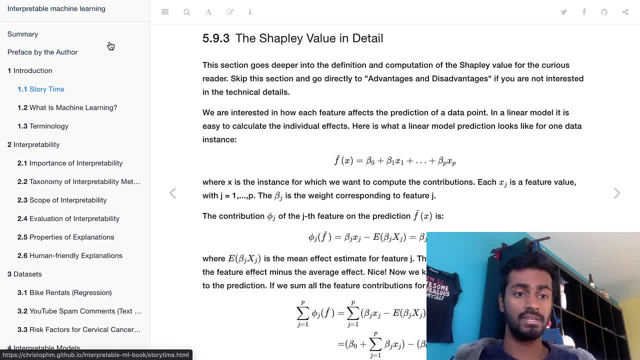 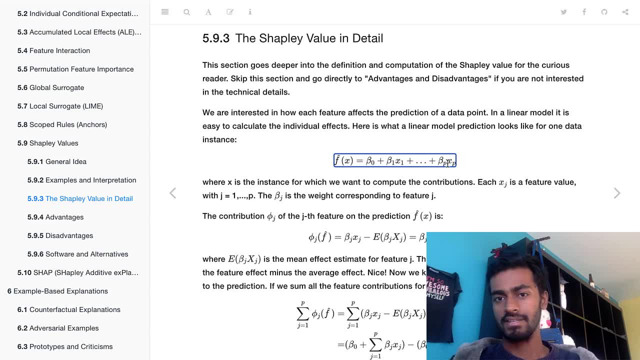 like interpretable machine learning. I honestly recommend you to go through this. It's a great read with a lot of examples and also lots of good mathematical detail. So let's say that we have this model right. It's a linear regression model. for now. 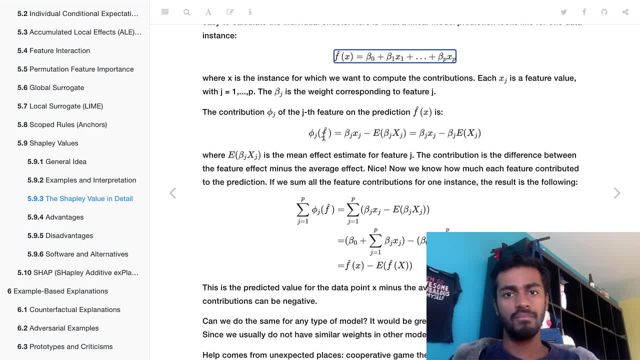 F of X right, And we could determine feature importance here by just taking the effect of the model minus. the effect of minus like the expected value of that feature, And I know there is, like some and if you aggregate it across, all like features right here of a particular sample.